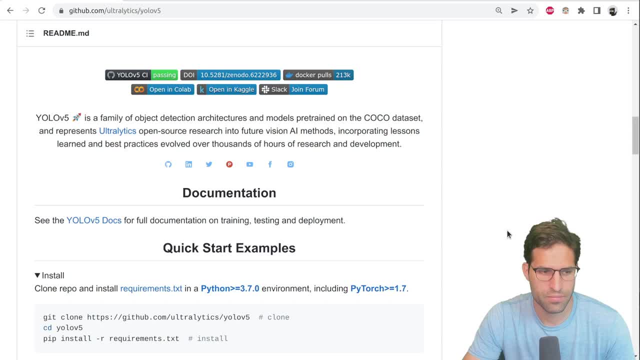 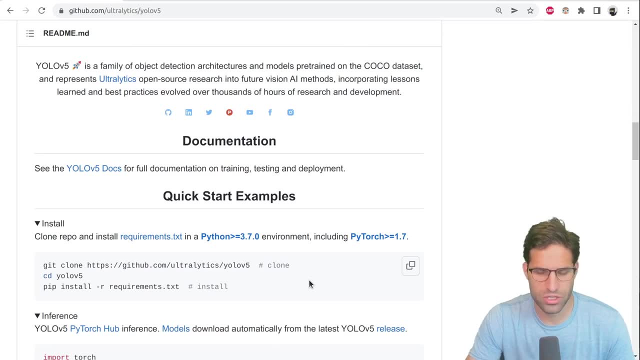 what they do and what they aren't doing, So you can see- they're just working at the same time- what it is and have some official documentation To get started with it. the first thing we actually need to do is clone this repo. Now I'm working on my desktop machine, which is a Linux machine. 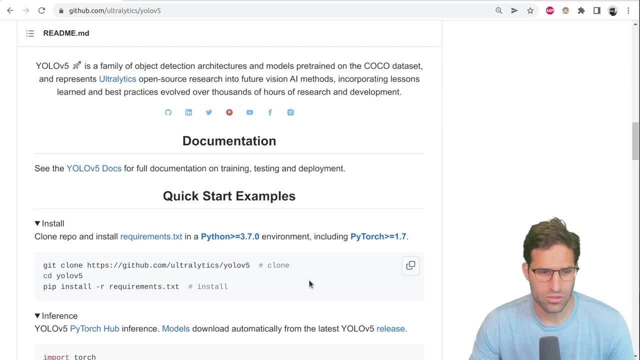 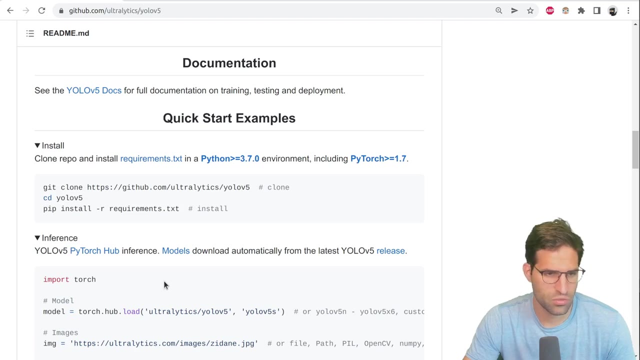 running Ubuntu 2004 and I also have two GPUs in this machine that the YOLOv5 will use to predict. It also uses PyTorch as the back end, where all the models were trained, and we will actually set up a new environment here that will run YOLOv5 and have all the correct packages installed. 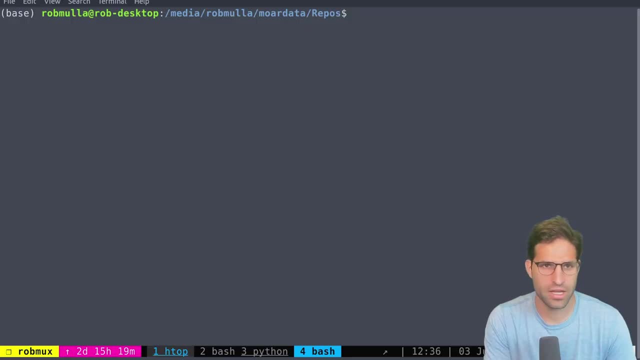 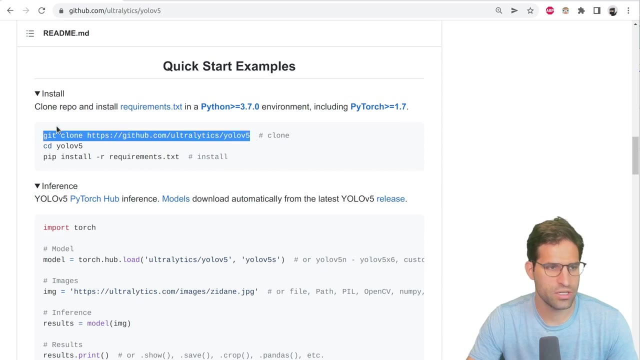 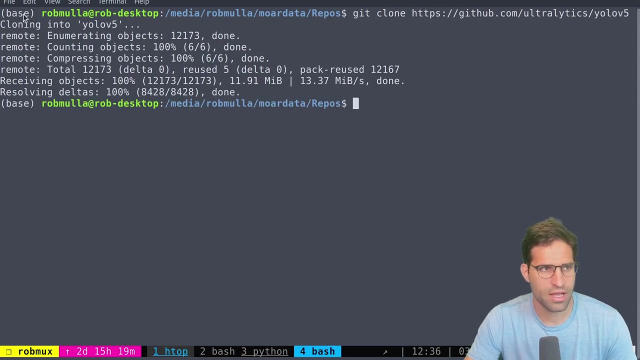 So I'm switching over here to my handy terminal and I'm in my directory where I like to clone my repositories, and all I'm going to do is run this git clone here Now. it's recommended, too, that you have Anaconda installed Right now. I have Anaconda installed on this machine, and that'll let me. 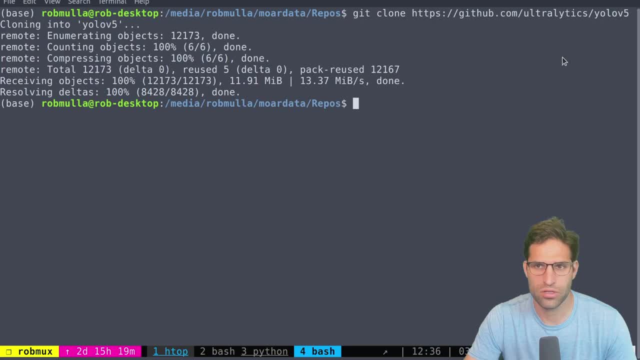 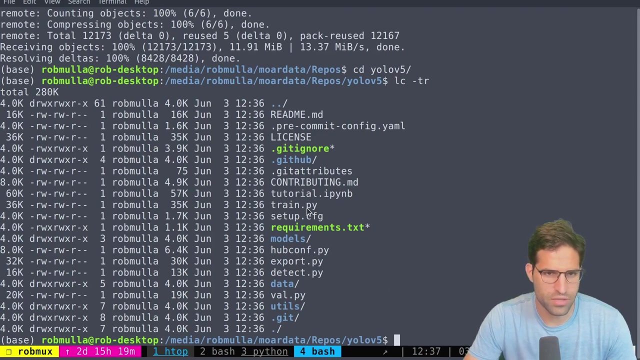 create a brand new conda environment for YOLOv5.. So what it says to do next is just to cd into this directory where I cloned and if I do lctr, we could see: these are all the files from this GitHub repository that we have cloned, And then I'm actually gonna. 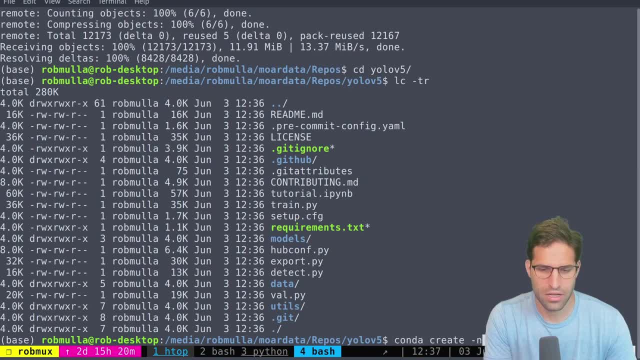 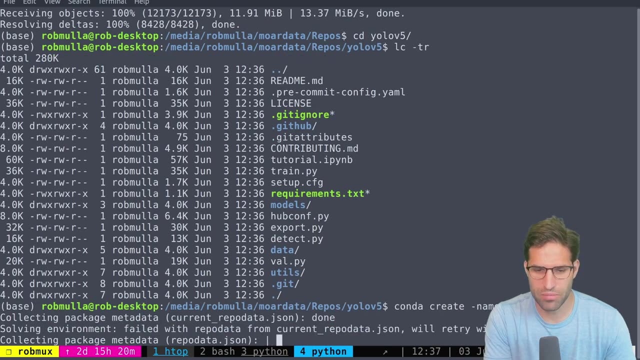 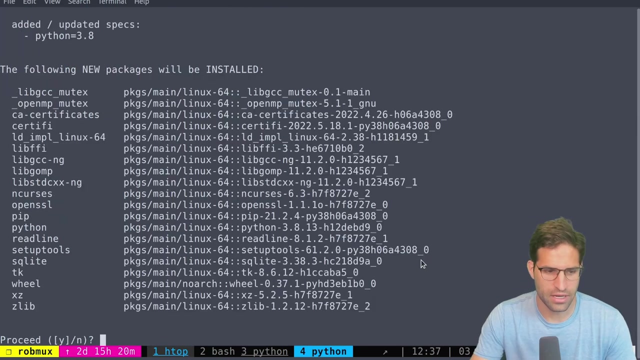 Anaconda create with the name YOLOv5.. So I'm going to create a fresh new conda environment where we can install all the required packages. So I just do that by doing conda create dash name. I named it YOLOv5 and I do need two dashes here in the name And I'll type yes to install all these dependencies. 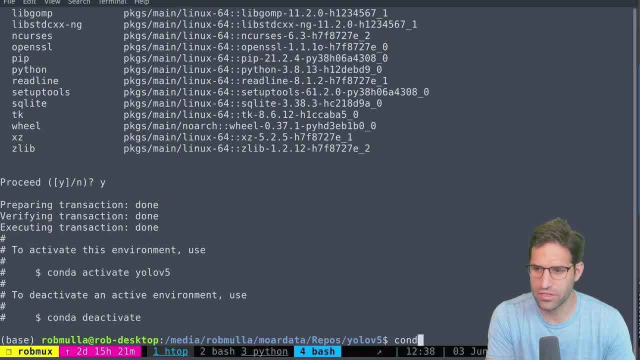 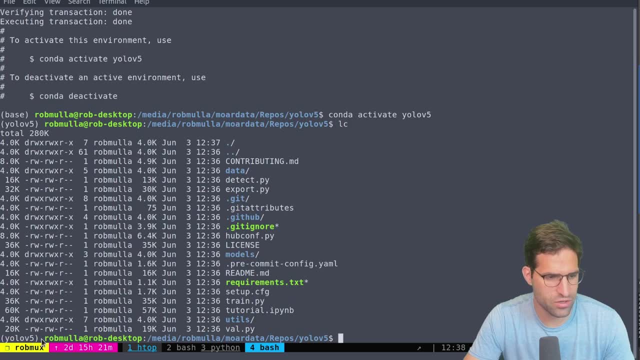 Okay. So in order to activate this conda environment, I just do conda, activate YOLOv5.. Activate it in this environment and you can see, because it says YOLOv5.. I also made sure I installed Python 3.8 because 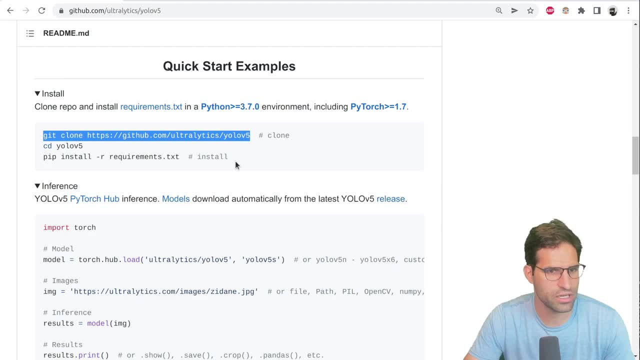 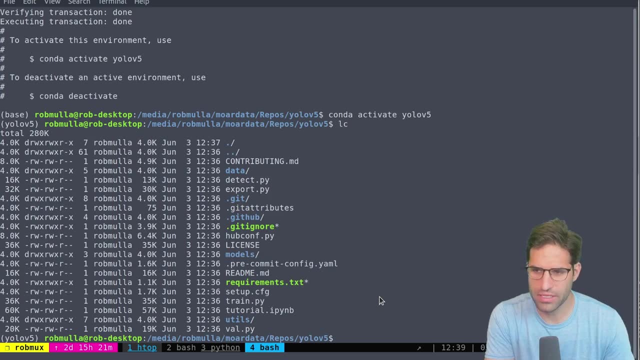 the docs for YOLOv5 do say it needs at least 3.7, it looks like. So now that I'm in here I can just pip install all the requirements that are in this requirements text. If you want to just look in the 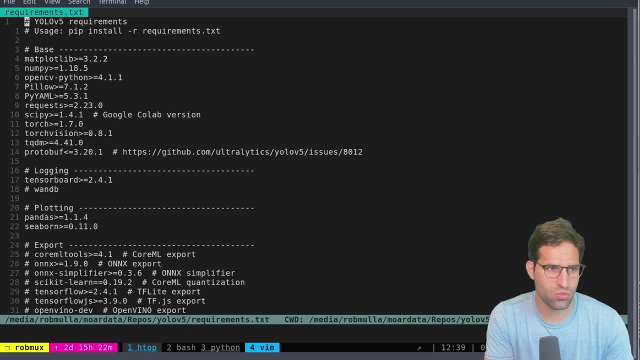 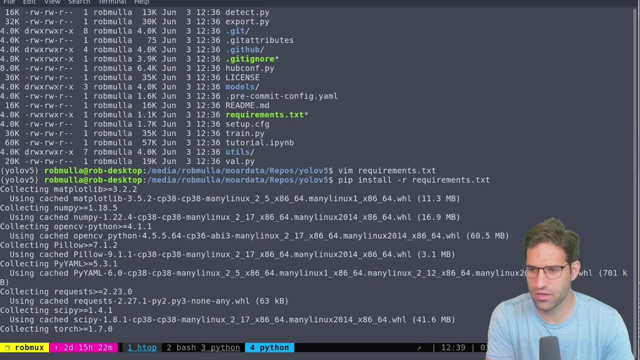 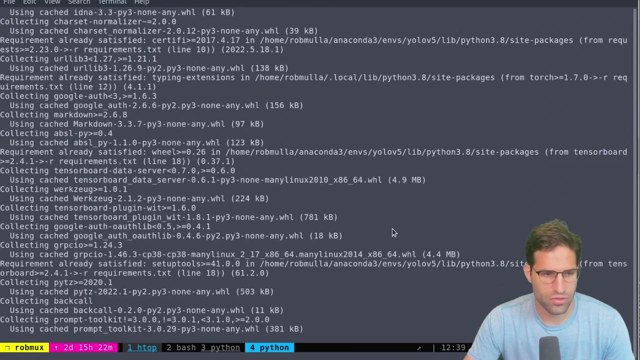 requirements text. these are all the packages that it will install and it will make sure I install all the right versions. So this might take a little while because it's going to have to download some of the wheels if it's your first time installing these packages and it needs to run through and install them all. Okay, so it looks like. 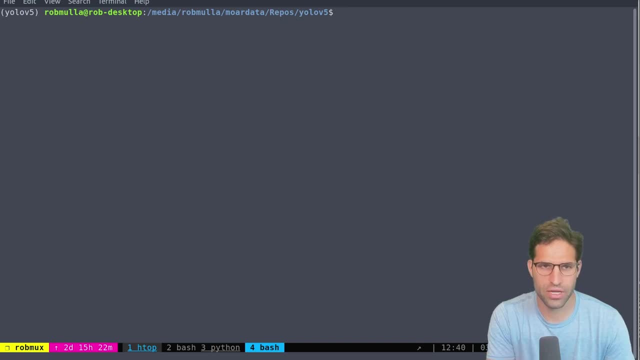 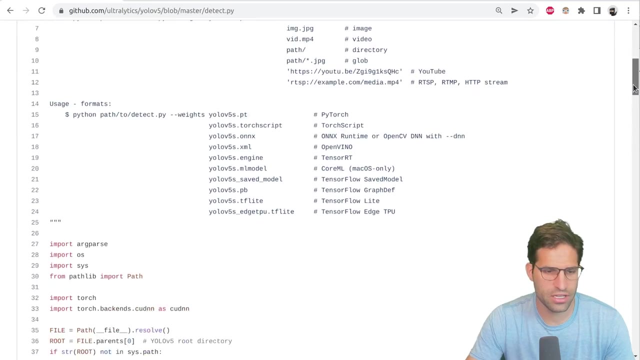 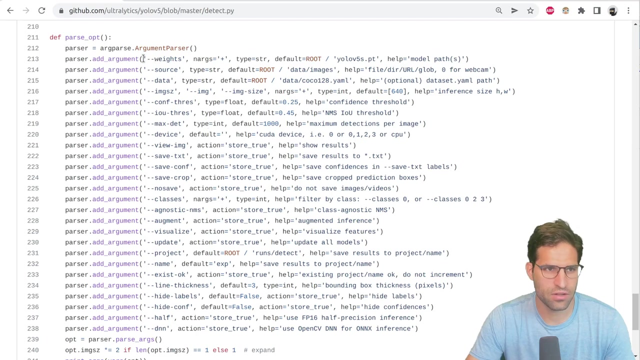 it's done installing them all. So I'll just clear this screen. If you look over in the repo in this detectpy we can see it's actually can be called just from Python with some arguments. So by default it will pick certain weights to use, So YOLOv5. 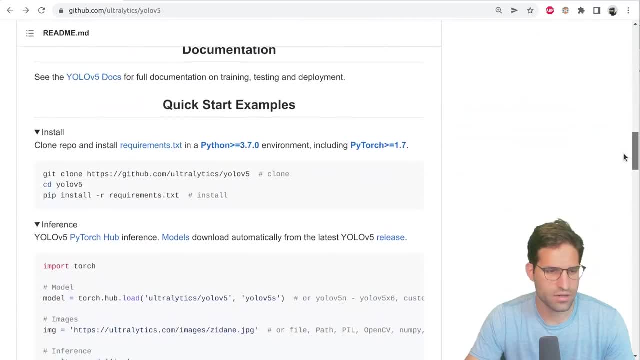 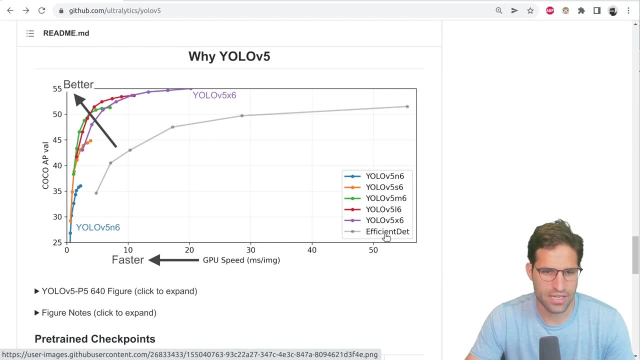 comes in different sizes. Let's look and see what size is of the weights that we have as options. Yeah, so they're shown here, YOLOv5.. The smallest is n and the largest is x, and it looks like there's even a new one efficient debt version of it, And 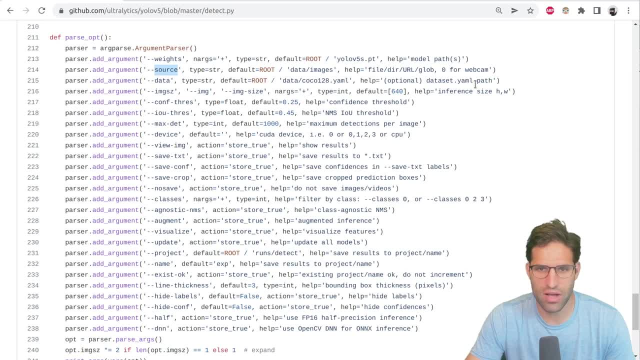 what else are we going to get it? We're going to need to provide it the source. Now I want to provide it this: my webcam, to see if it will run directly on my webcam. and we just provide the number where the webcam is associated. So if you only have one webcam, you'll be putting in. 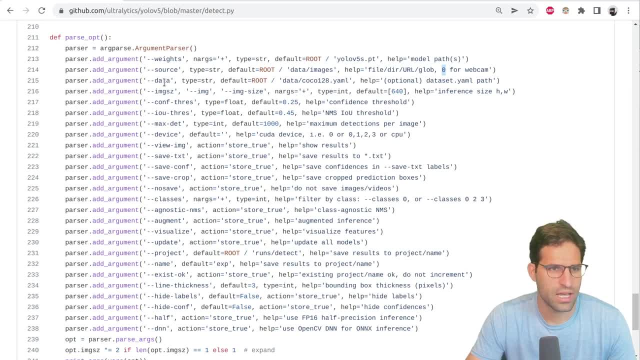 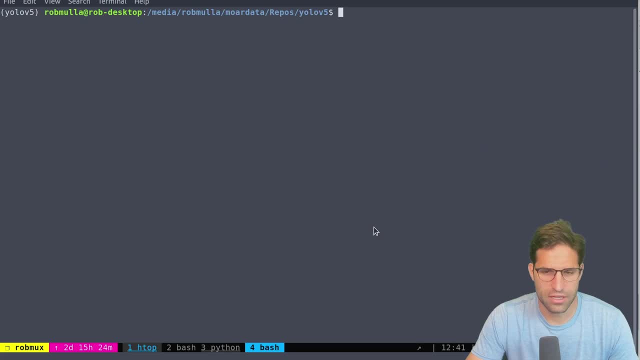 zero here and we'll see how that that works, And we're not actually providing any data to train on, so we don't have to worry about this. That's all we really need, I think. Okay, so I think I have it working Here. the command that I needed to run was just Python detect, and then I'm using source five, which is my second webcam, and I have a green. 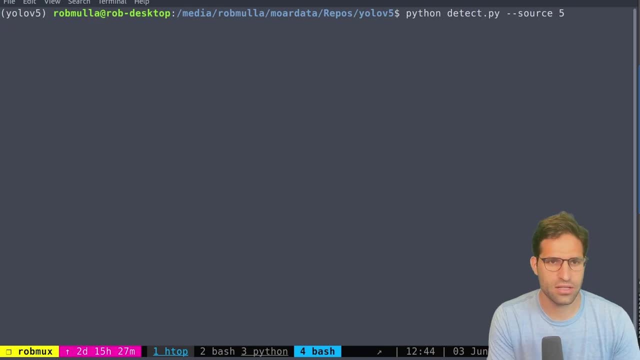 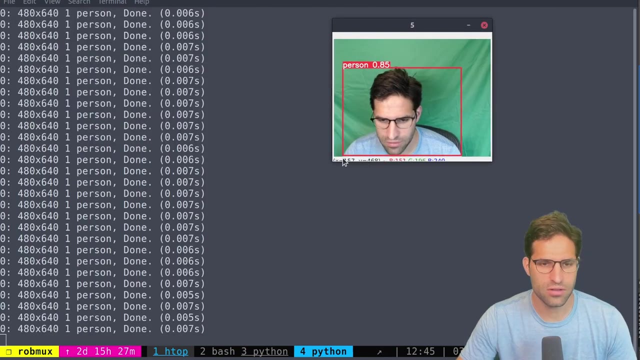 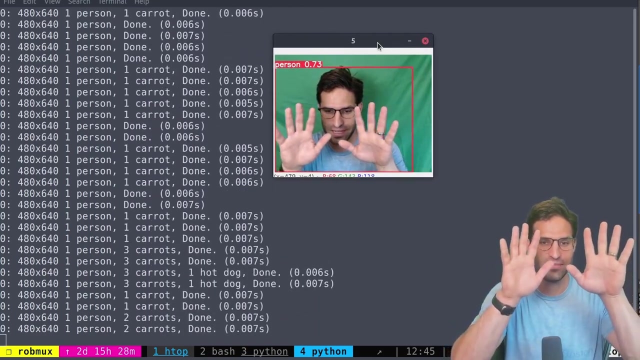 screen here behind me, so it's going to show the green screen when it loads up. Let's try running this detect and see how it works. We can see that it is using the small version of YOLO weights. but there we are. So you can see me. there's a person. Here's my- Oh, it thinks my fingers are. 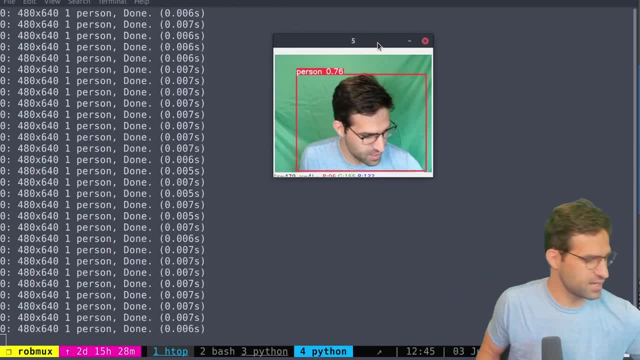 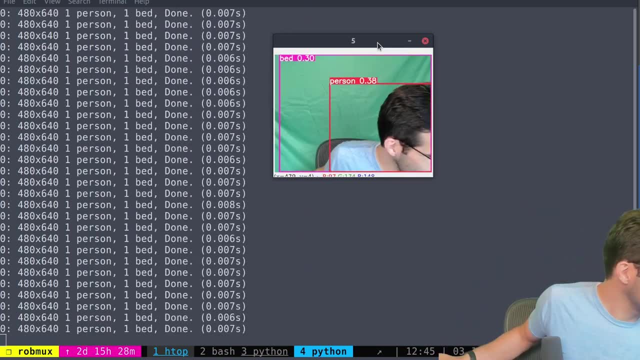 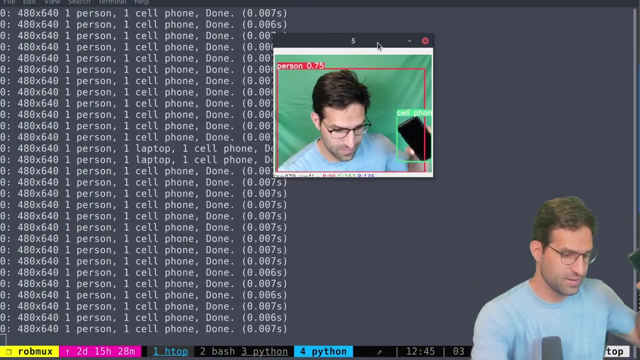 carrots. Thumbs up, Let's hold up. Let's take off my glasses, No glasses. Tennis racket: All right, Not perfect, Not perfect Phone. Cell phone- It's good at that. Maybe a cup Cup- Okay, Yeah, that's pretty good. 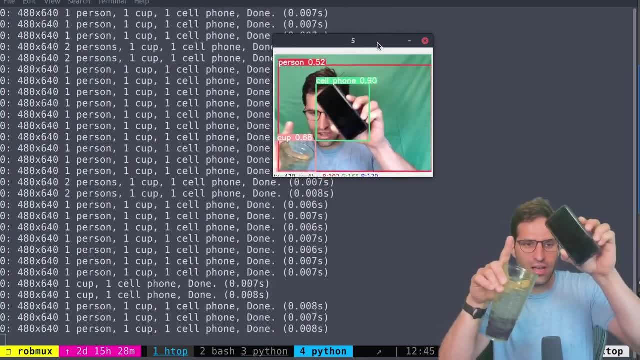 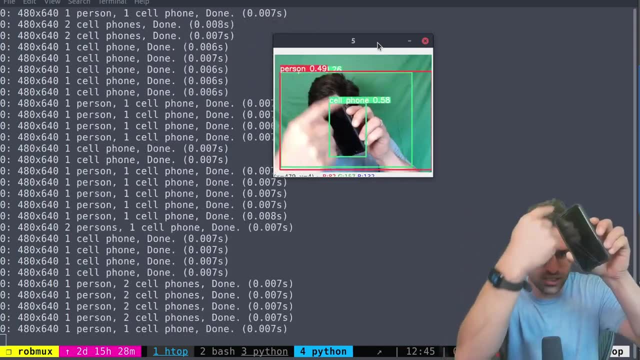 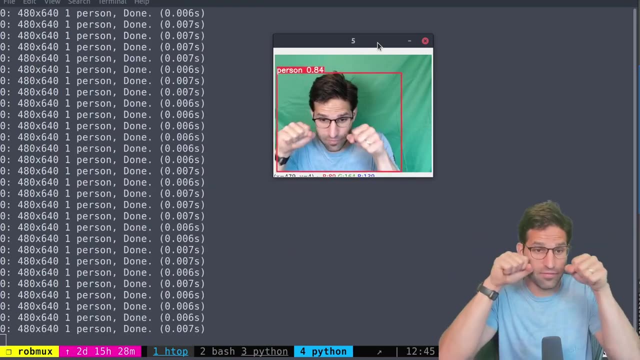 And you can see the confidences are shown on the side of the image. So it's drawing the bonding box and showing the side. But if you wanted to pull out just the bounding boxes, you could do that as well, Or store any information from YOLOv5 by. 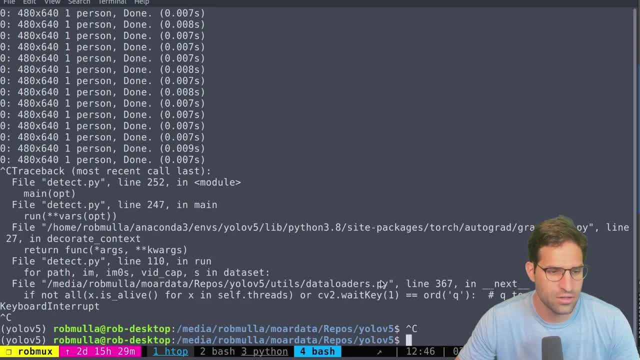 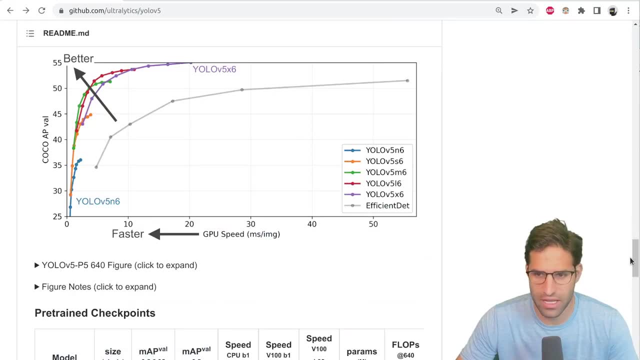 going into the source code, Cool. So we're going to kill that and let's try to load the larger weights, because the larger weights are going to mean that it performs more accurate and it's might be a little bit slower, but it's going to. 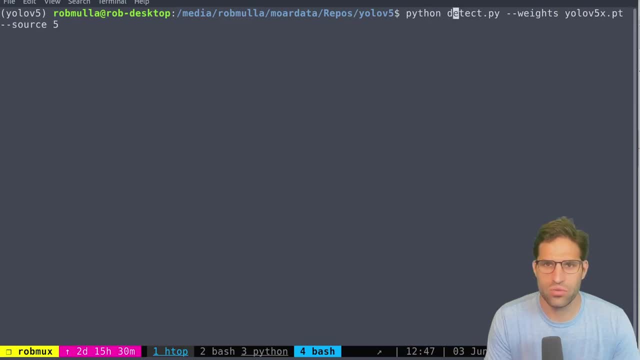 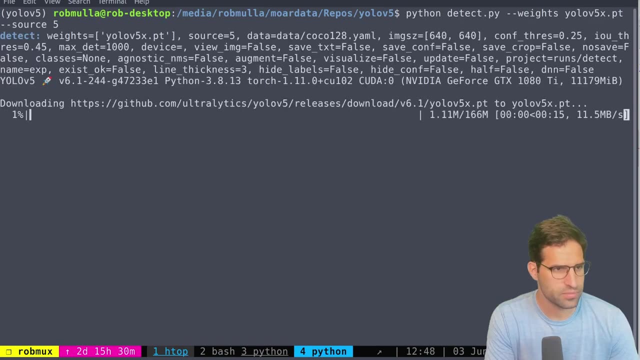 perform better. So what we need to do to get the larger weights is run Python detect and then feed in the YOLOv5x weights and then give it the same source. Now you can see it's actually downloading these weights, Fusing the layers. 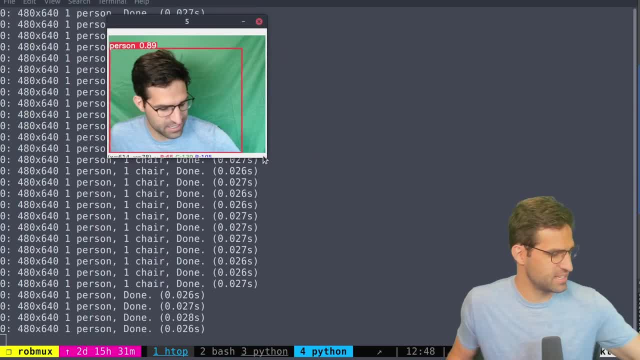 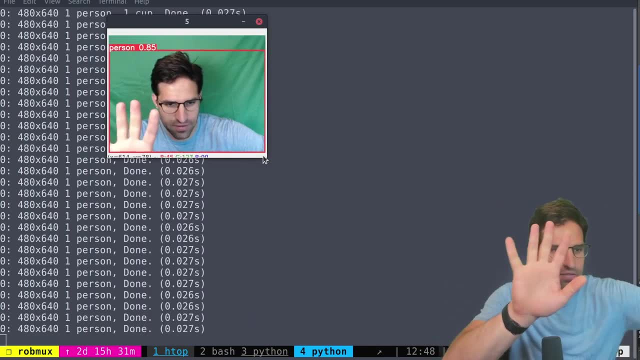 All right, And now we're back to my object detecting. It can see the chair, It sees the corner of the chair. It knows this is a lot better. Does it think my fingers are still? No, It's pretty good about my fingers. 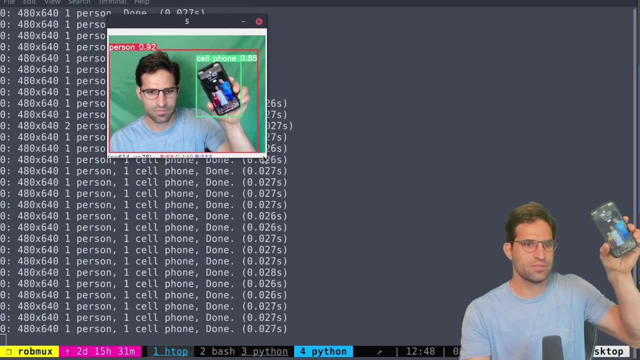 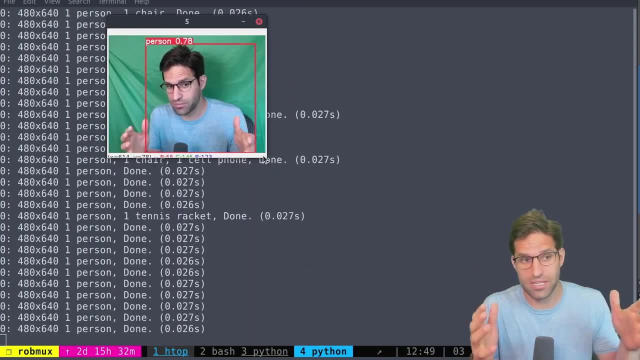 Maybe if I just hold my hand. No, it thinks I'm a person. Cell phone: This is just working on the default pre-trained weights. but if you wanted to, Does it know? this is a microphone, But you can make it more customizable by fine tuning. 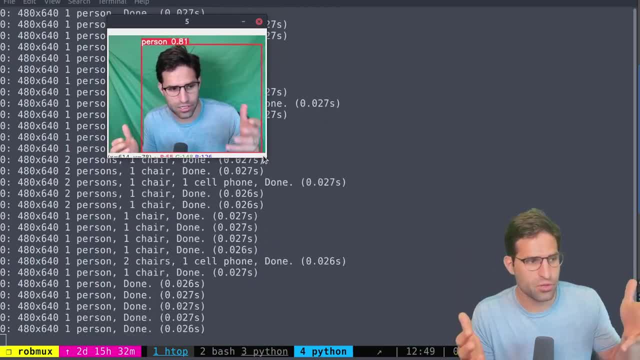 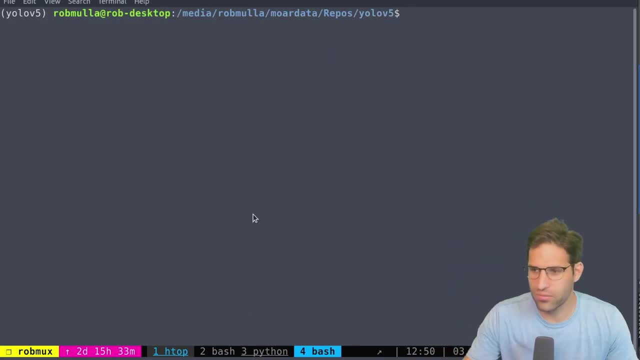 the training on a different data set that's pre-labelled. There we go. Look, that's pretty good. It's pretty confident of all the things. Now let's try to run it on video data set. So I do have this data set, which is a. 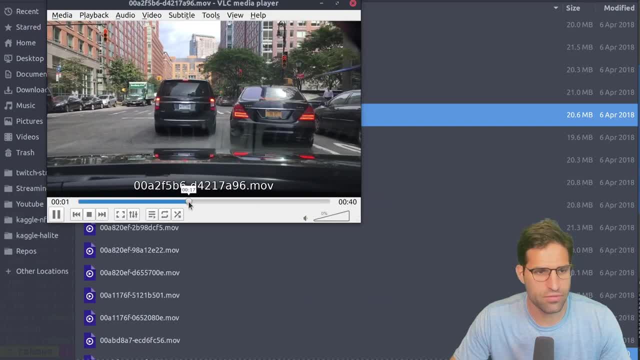 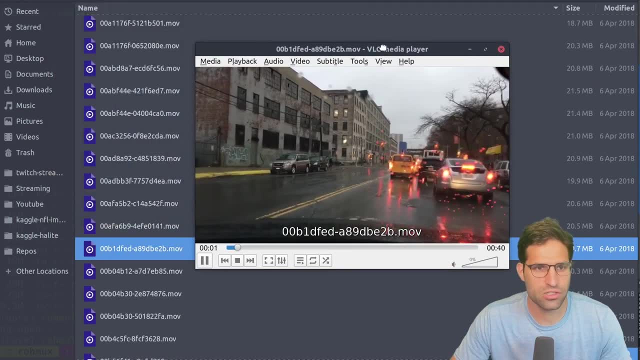 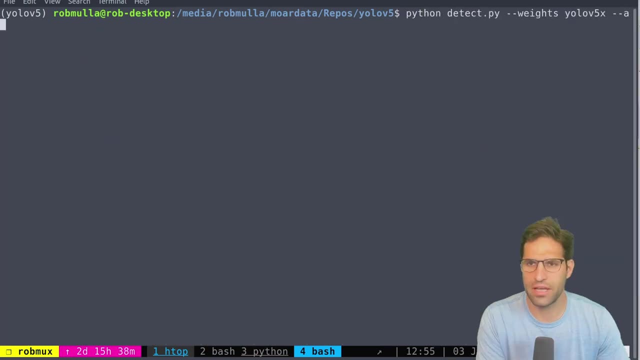 video footage of a bunch of different cars driving around and I'm using this for a different YouTube video that I created on working with video data. But let's try to run this object detection on this video and see how it works. We're going to call this again. 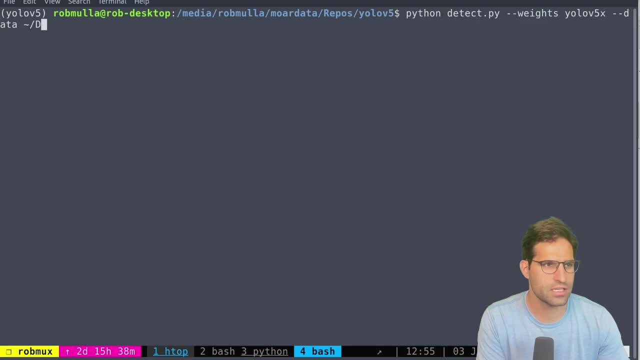 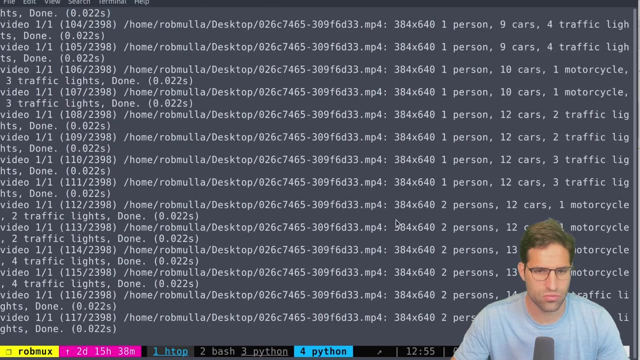 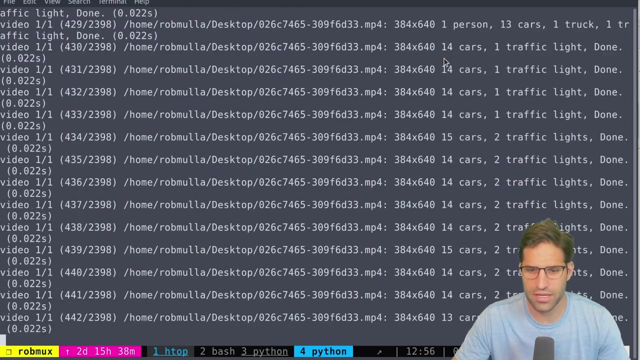 but instead of giving it a source, we're going to give it the desktop mp4 file. Okay, so it looks like it's running and it's detecting people, bicycles, cars- So what it's doing here is it's running. now, on this data set It. 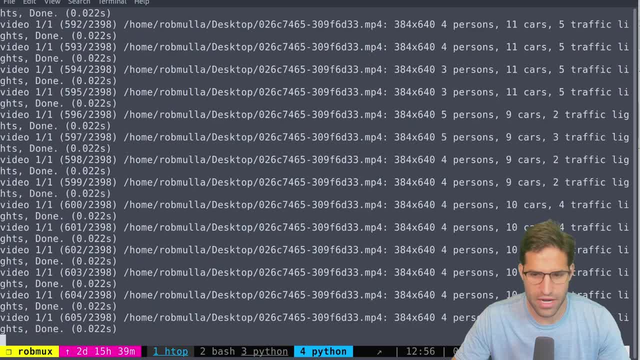 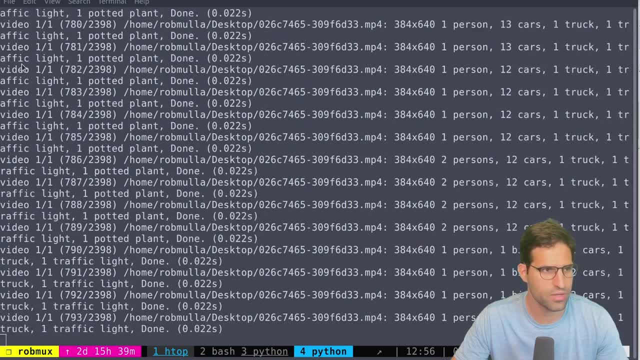 has the number of frames that it's gone through of the entire video and the number of people that it sees cars. These are just some of the labels coming out here, printed to our command line So it looks like we can provide it view image. 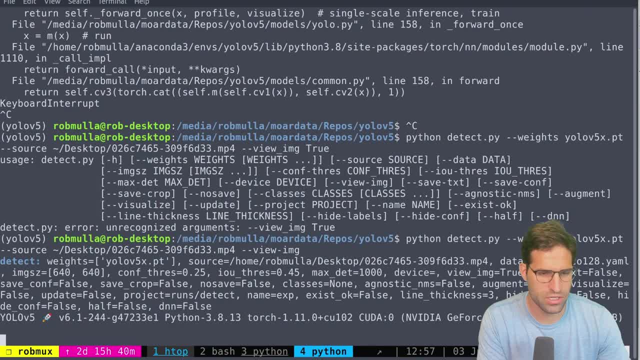 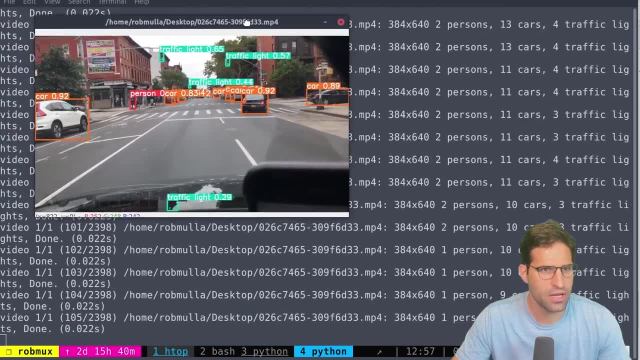 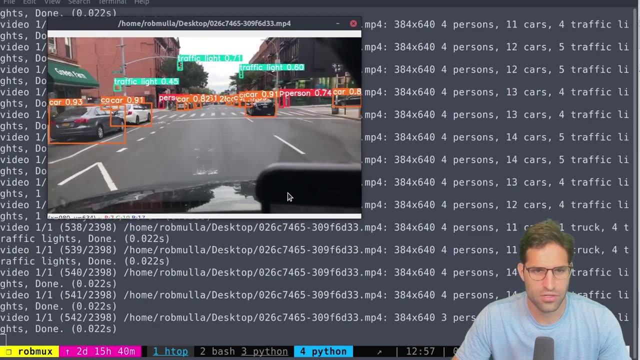 like this in order to actually view the images as it's processing. Yeah, there we go. It's a little bit slower, but it is working. We see that it's detecting all these different cars and objects, even detecting the traffic light, which is really impressive. 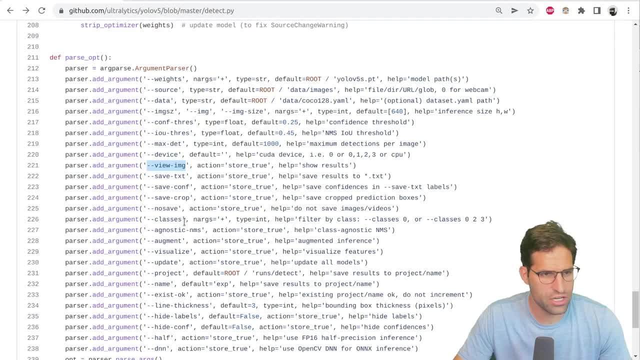 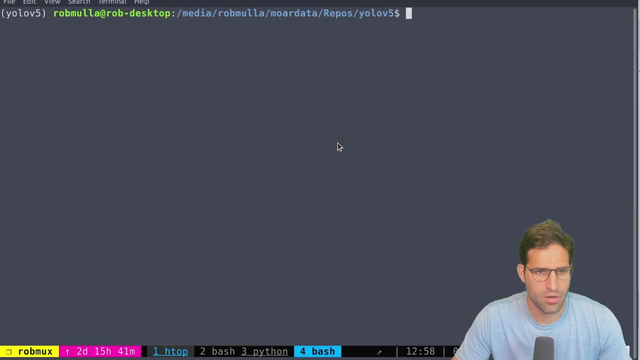 So if I kill this now, I can change other settings like the confidence threshold and the IOU threshold. So if we only want it to show objects that it's very confident of, it's defaulted to .25, but let's change that confidence threshold to 0.9. 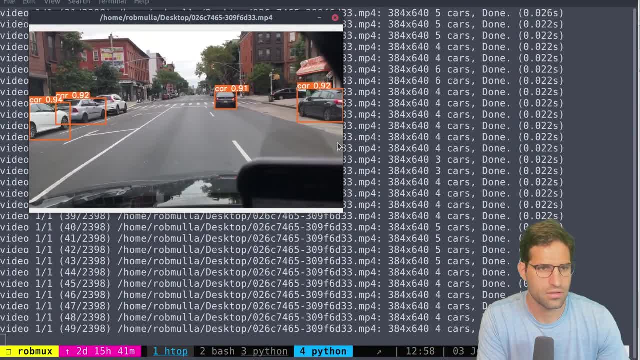 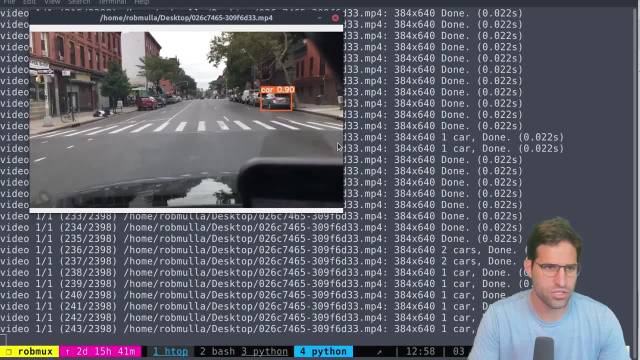 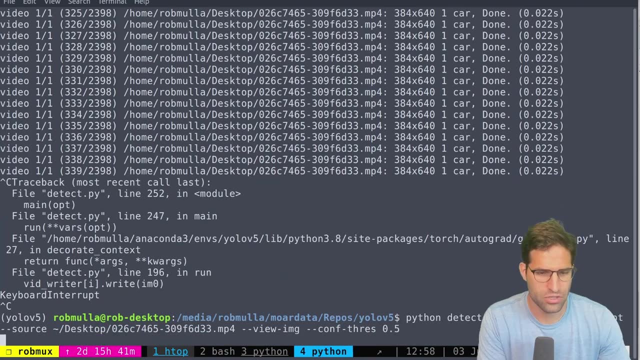 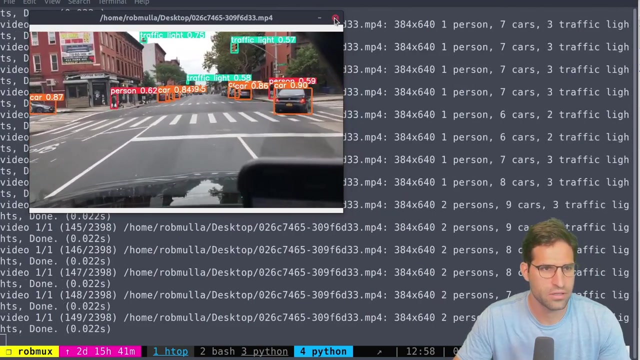 and run that There. now it's detecting much less, because the threshold that it needs to detect in order to show needs to be at least .9.. Let's do .5. Okay, that looks pretty good. And then there's also something called an IOU threshold. 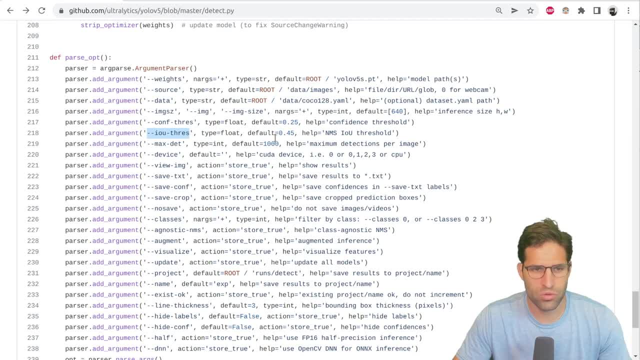 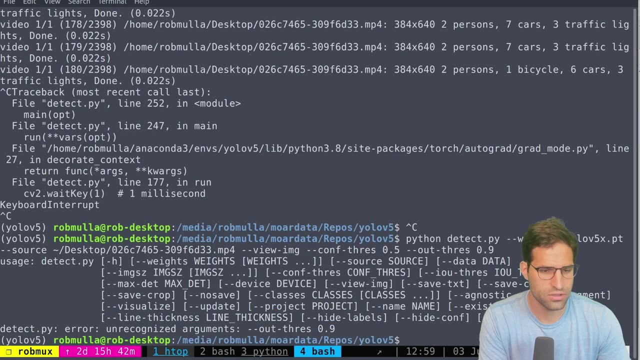 and this basically means it will suppress any objects that it detects that overlap each other. So IOU has to do with the overlapping of two detected objects. Let's do .9 for the IOU threshold 0.5. So what's happening here is when we set. 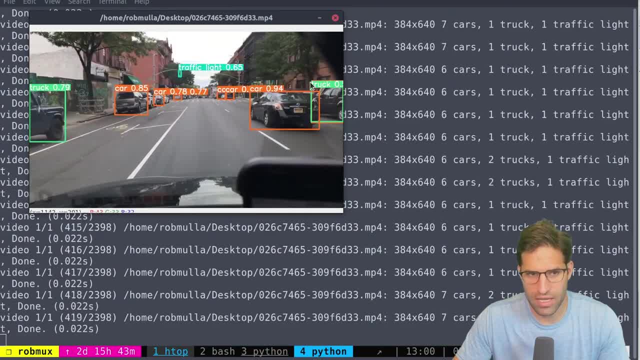 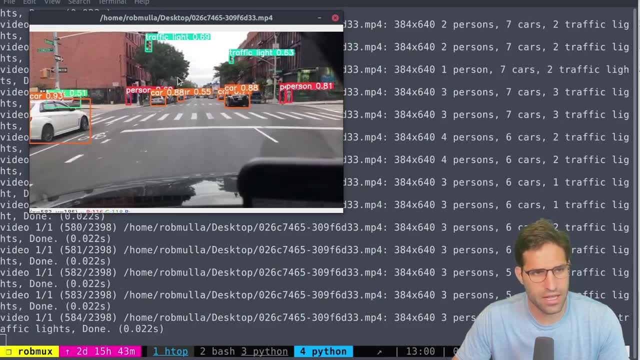 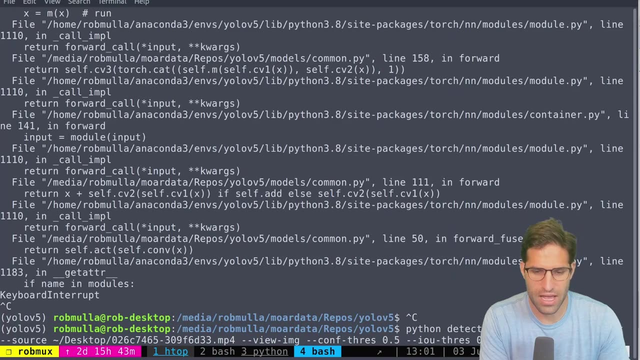 the IOU confidence to be really low. it won't allow any boxes to be overlapping each other very much. It'll just suppress any object detection that overlaps with another object detection. So by turning this off and setting it really high will allow for a lot of overlapping. 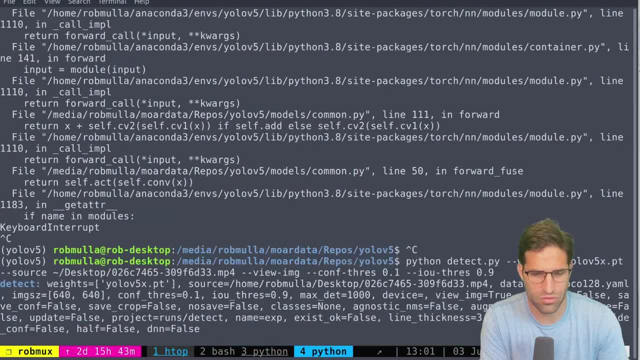 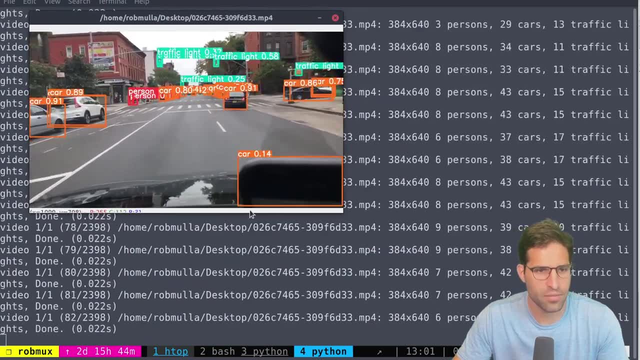 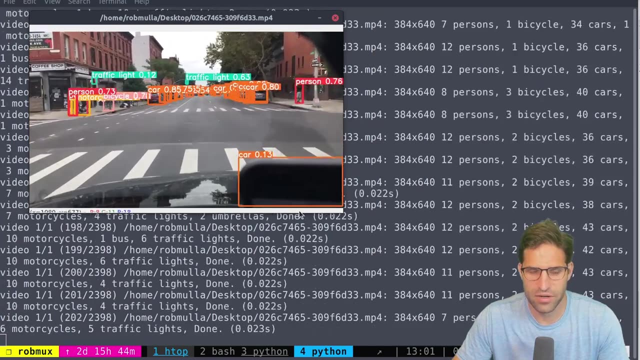 boxes And let's do one last run with a really low confidence threshold and a high IOU threshold. There we go. So this is a lot of different boxes and even this car that it's detecting in the lower right side is very low confidence, but it's displaying it.